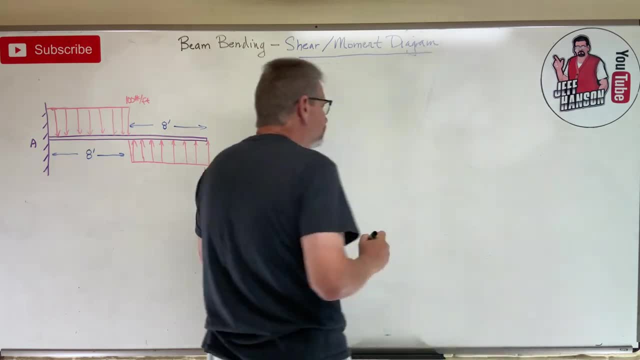 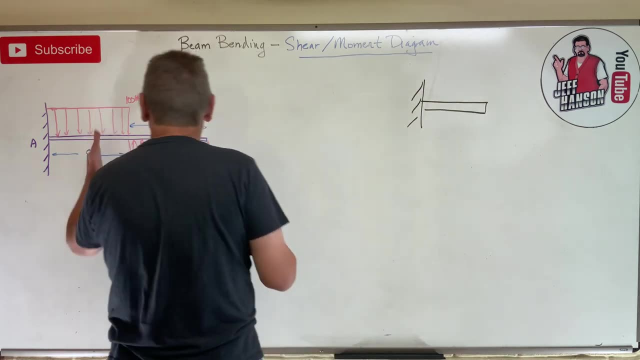 like you've never seen it before and here it is okay. So remember when we did before, when we said: if you take a beam, if you cut a beam in half, you section it at some point. okay, You have these. 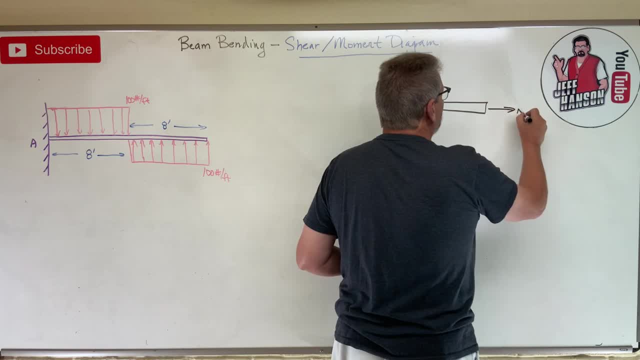 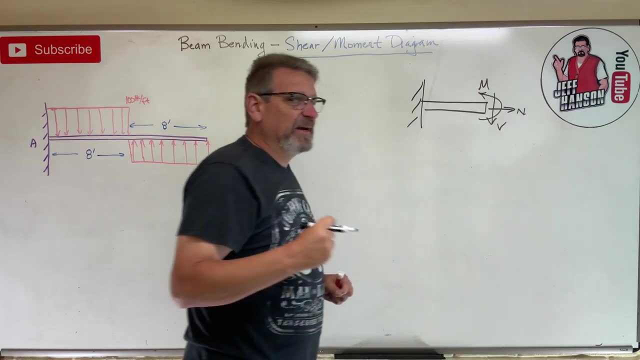 internal forces in the beam. okay, You have an N, a normal force, You have V- a shear force, and you have M, a bending moment. Now, we've already covered that in another video. Remember every time you cut the beam. 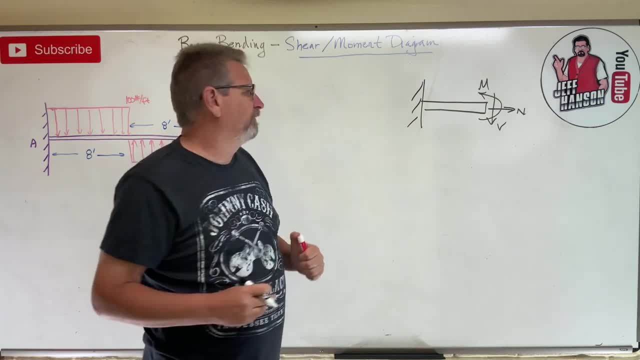 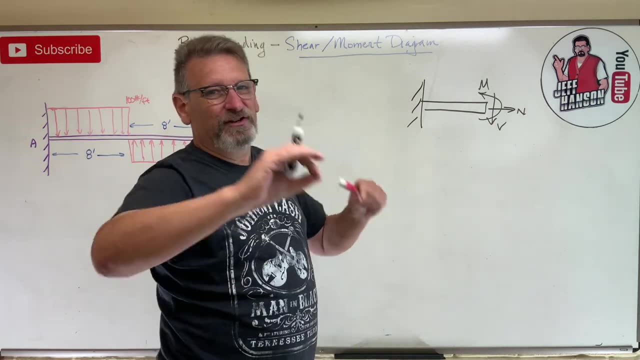 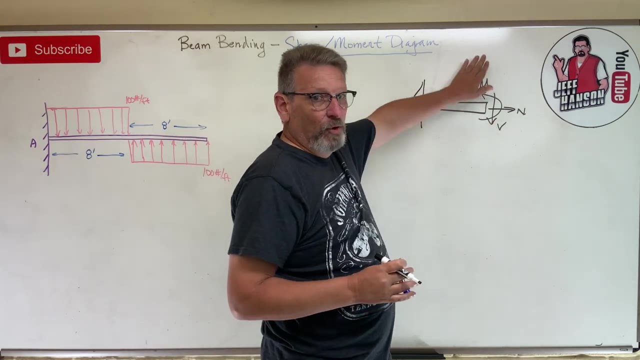 you must have an M and V, You have to sit in Mickey Mouse voice, okay, But we could go back from the last video. we could determine M and V, those internal forces, at any point on the beam. But what if we want to know, like M and V, the moment and the shear? 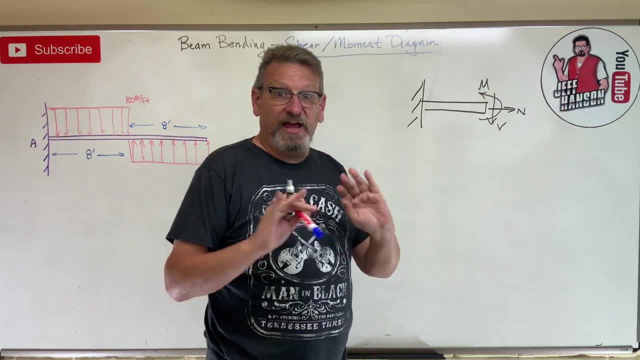 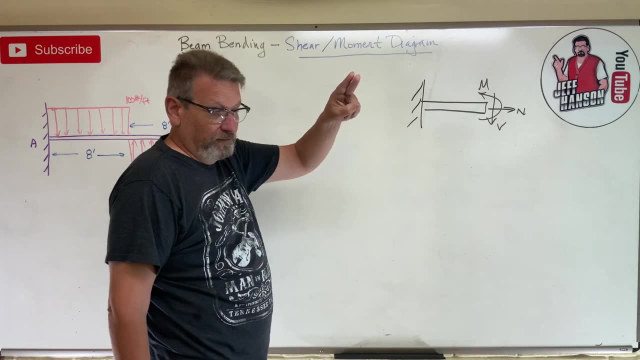 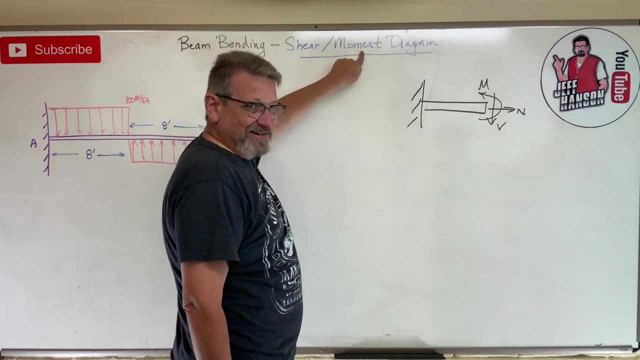 at every point on the beam, not at a specific point, but every single point. Well, we'd have to graph it, wouldn't we? And that's where we get shear. that's V shear scissors moment diagram. So this is the shear force, this is the bending moment. okay. 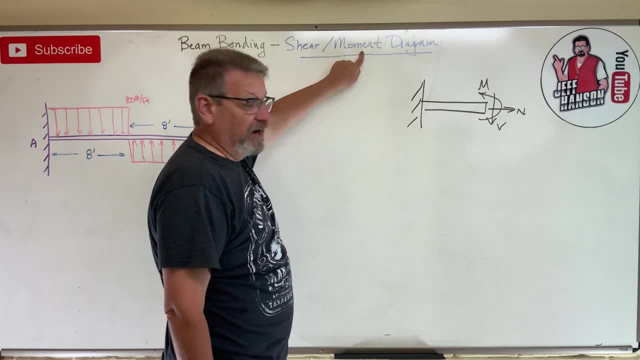 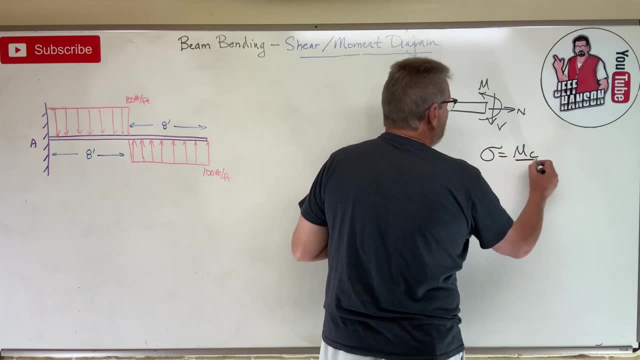 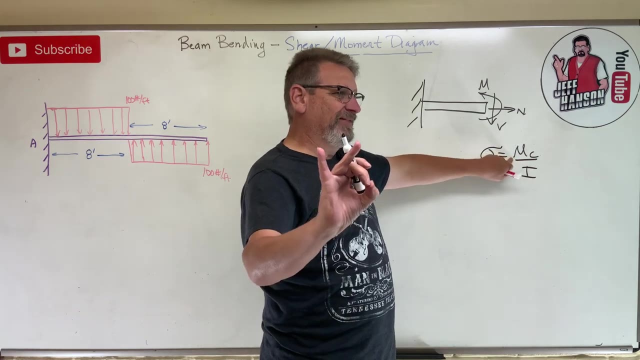 Now we need those things for some equations that are coming up. The big, the pivotal, most central beam bending equation is: sigma equals MC over I. It's called the flexure formula, and M is the bending moment. And where are we going to get that Off of that diagram? okay, So it's important. 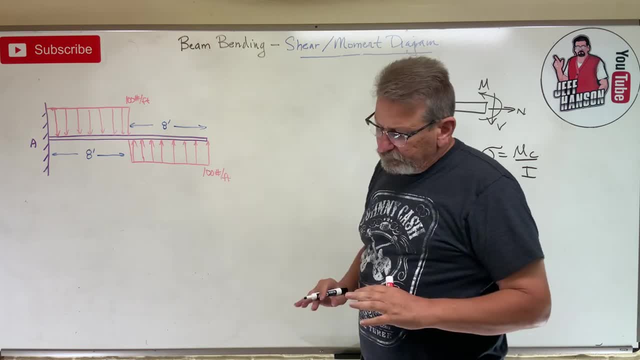 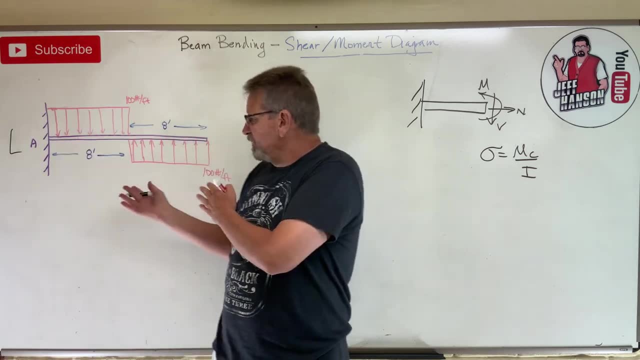 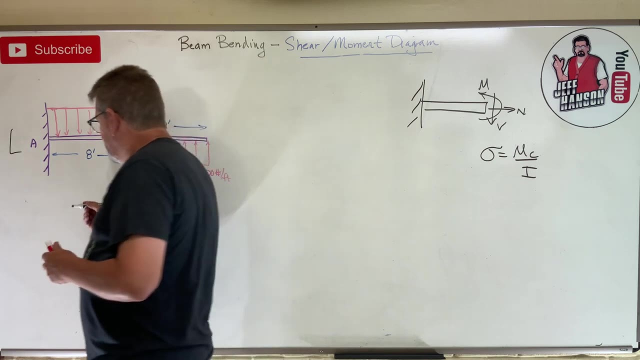 to learn how this diagram works. okay. Now, what I call this is: I call this L for the load curve, That's the given curve, okay? So this one's got two distributed loads, one going down, one going up. Don't mess that up, okay? And then what we do is we make sure we have plenty of room. 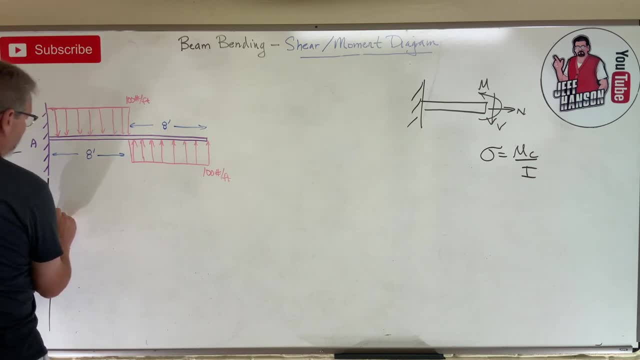 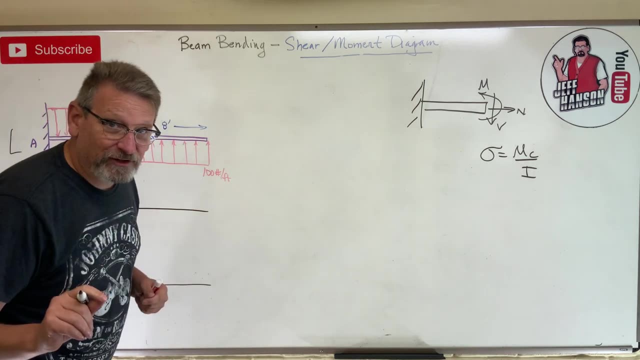 under this on our paper, because we have two, two graphs underneath this guy and newsflash a little farther on in the class. there's two more under this. There's the slope equation and then there's a deflection. So 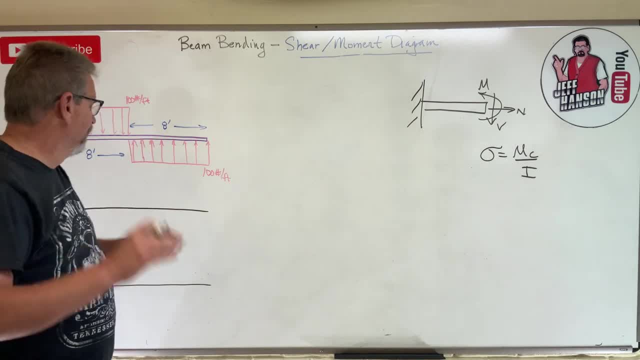 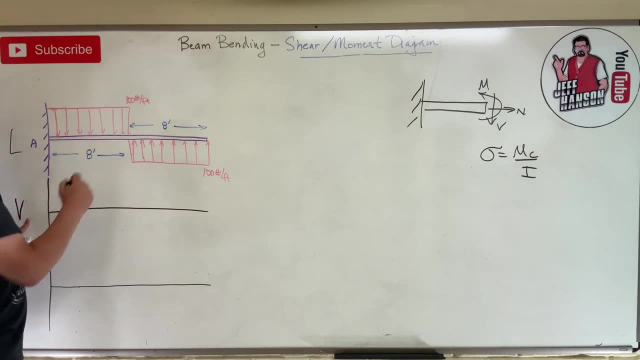 there's four integrals there. Oh, mind blown, We'll get to it, I promise. okay, And we call this one V. This is the shear force and in this case, with these units, this is going to be in pounds. 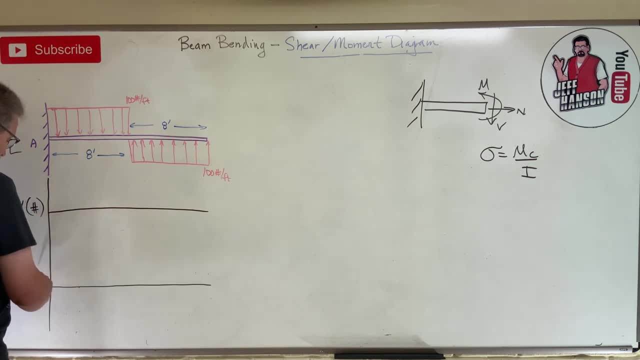 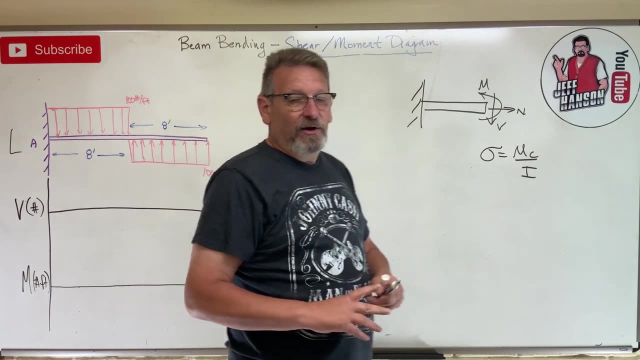 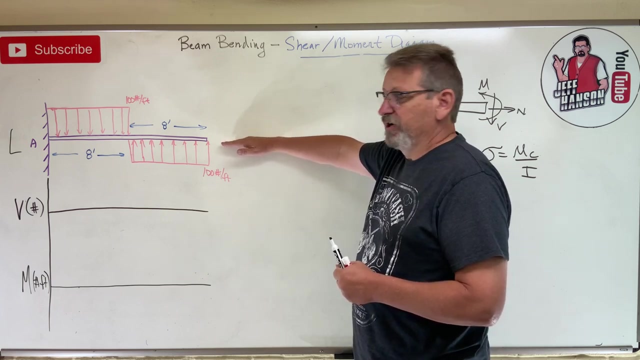 okay, And this guy down here is M the bending moment, and that's in pound feet. okay, Those are the units on that. Now these graphs are related to each other. The V graph is the integral of the load graph, So whatever functions define. 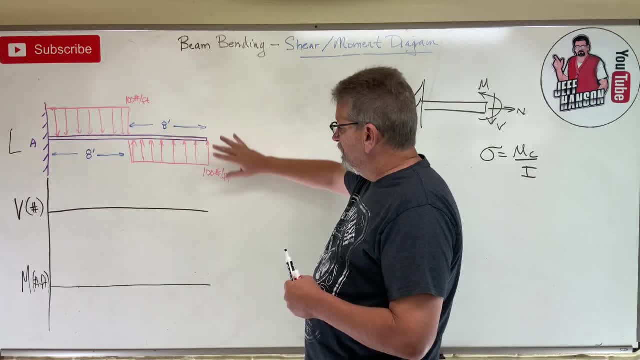 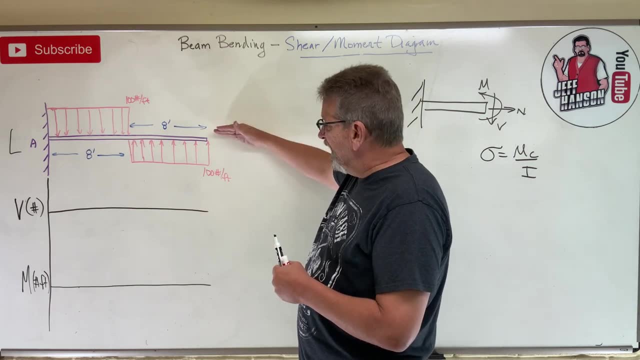 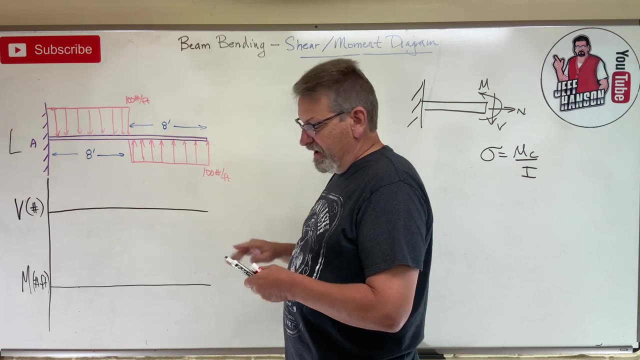 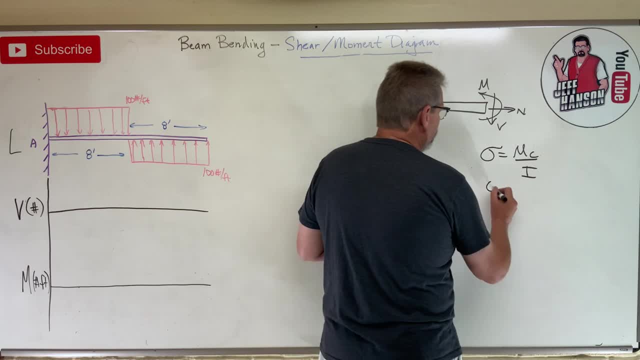 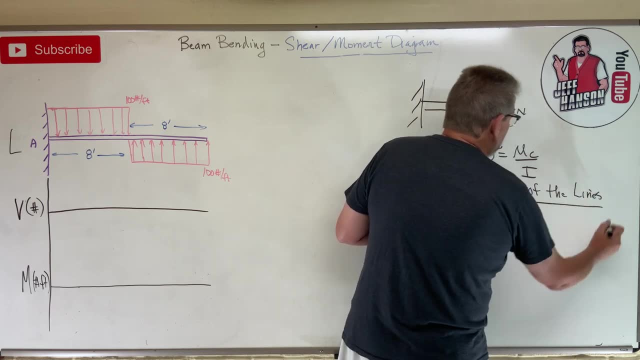 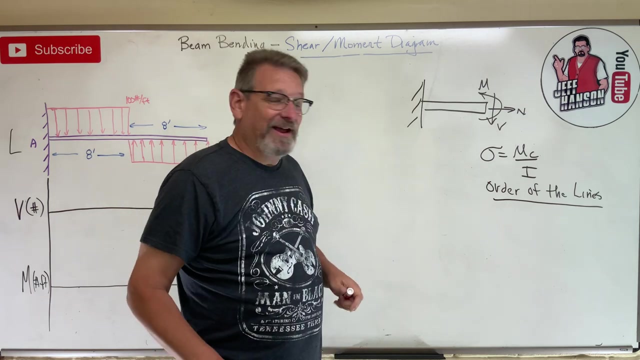 Now let me show you my little trick of the day here, and that is called the order of the lines. okay, Now, the order of the lines is not in any book I totally made it up. okay, Well, it's in one book: How to Ace Statics with Jeff Hansen on amazoncom right now. 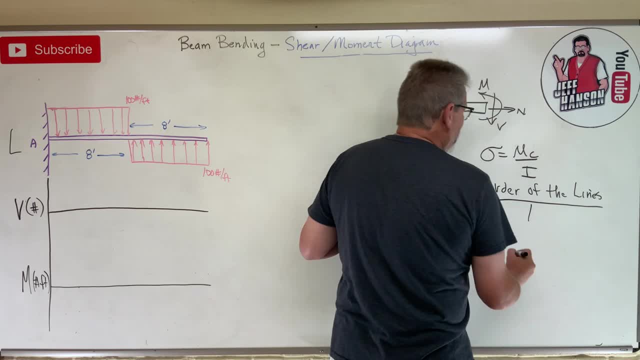 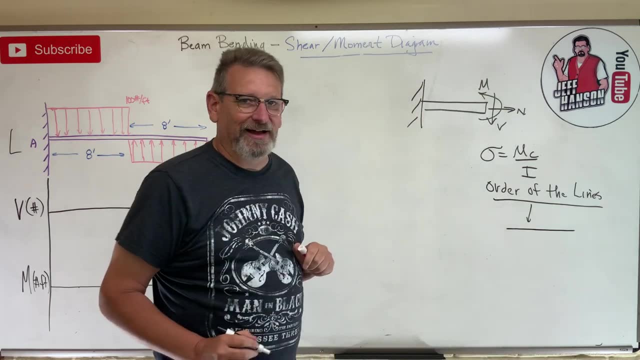 Go get you a copy, okay. So if I go straight down like a concentrated force, the next graph down is always going to have just a straight across line, a horizontal line That would be like y equals five, right, If I? 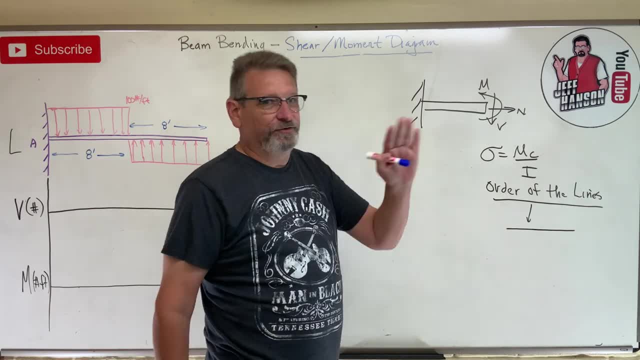 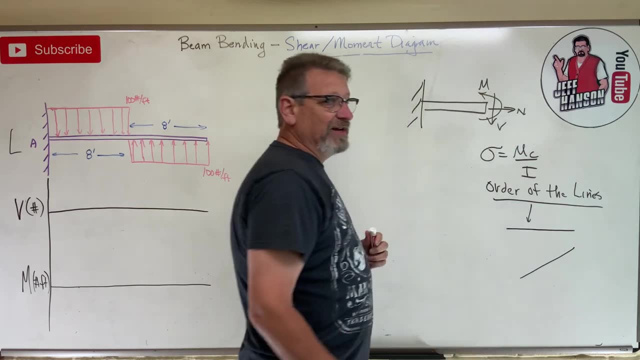 integrate that and go to the next graph down. integral of y equals a constant is what Y equals five x, right? So how do you plot that? Well, that's just a straight slopey-do, right. And if I integrate x, what do I get? I get x squared, which is: 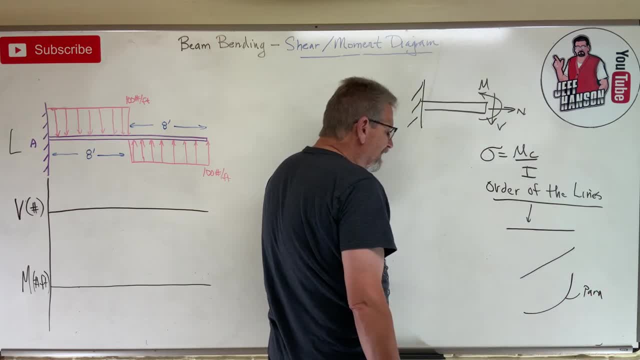 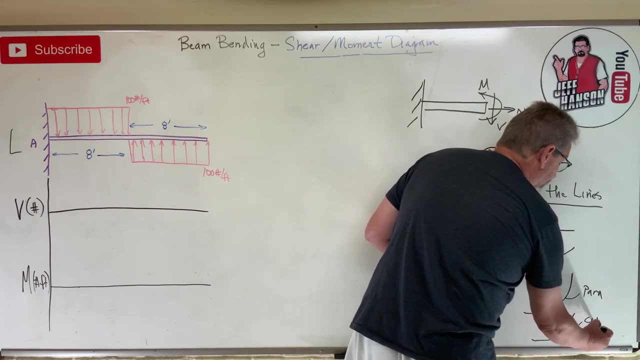 parabolic. I'm going to put a para there, all right. And then, if I integrate a parabolic curve, what do I get? Well, I get an x cubed, which we call a cubic. okay. So this right here tells me: 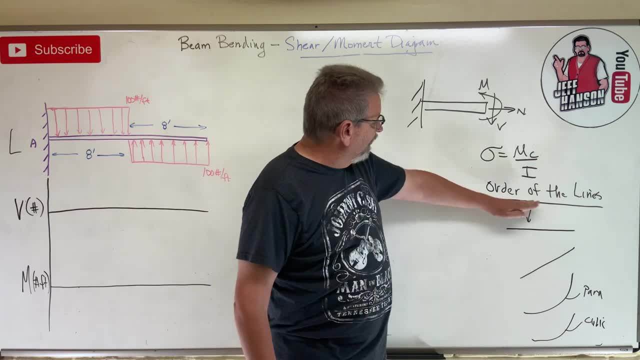 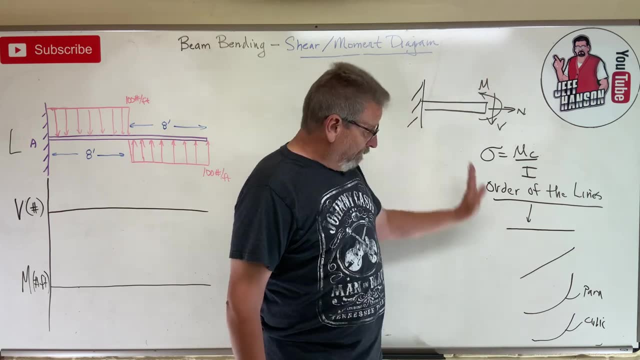 if I have that line on the top graph, then the next graph down is going to have that. If I have that, then the next graph down is going to have that. If I have that, the next graph, so on and so forth. If you can remember that- the order of the lines, you'll always get these shapes right. 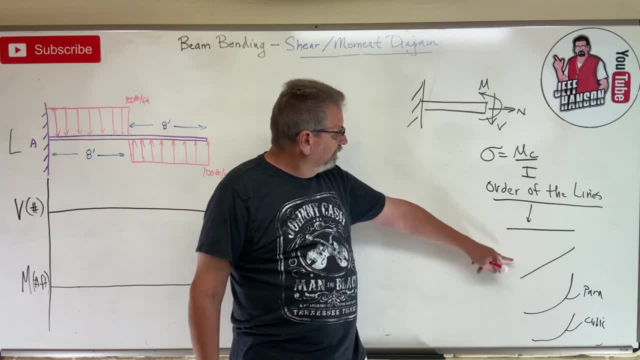 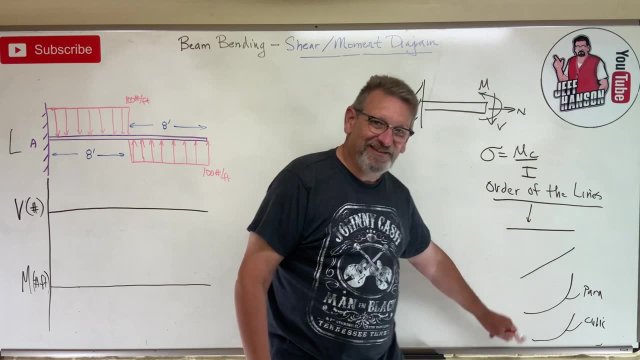 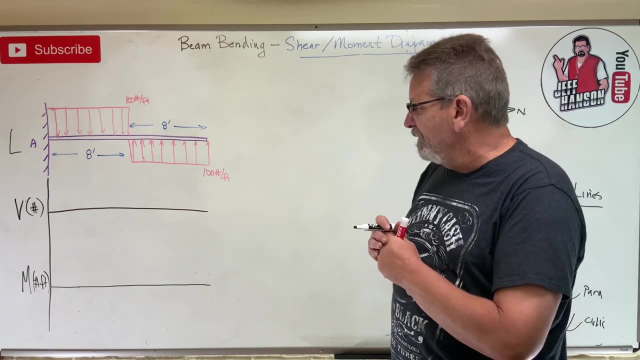 One has a straight across line, so the next graph has got to have a slope, which means that this bottom graph down here is going to have parabolic curves, right, All right. So if you understand that, you'll be miles ahead. So I think that let's see if we can solve this problem Now. 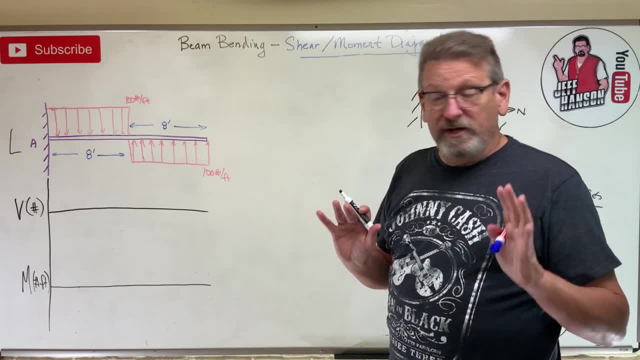 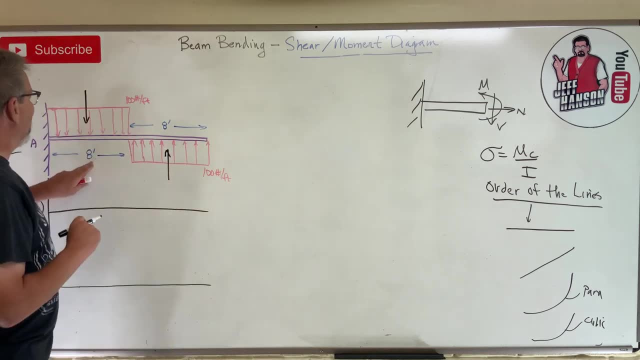 the first thing I see here is I've got two distributed loads. I want to turn them into concentrated loads by just adding a right one there and one there, And it's eight feet times 800 pounds per feet, So that's a total of 800 pounds. And this is a total of 800 pounds, okay. 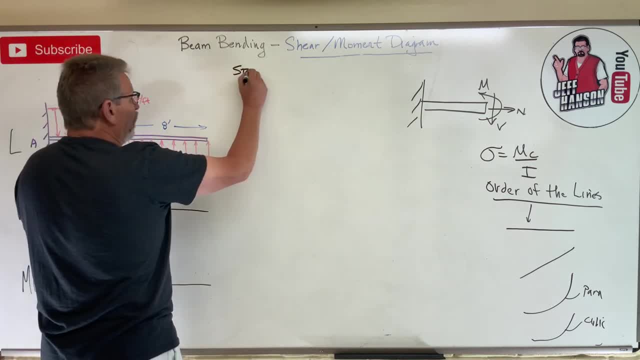 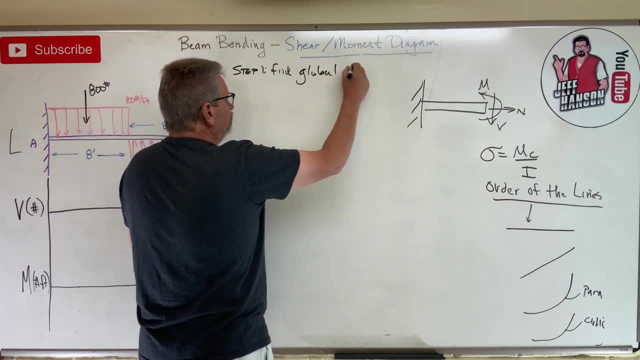 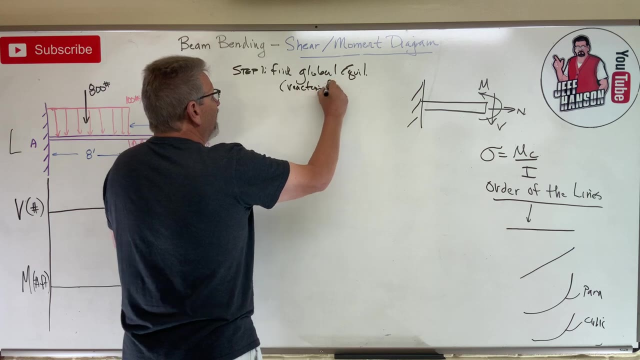 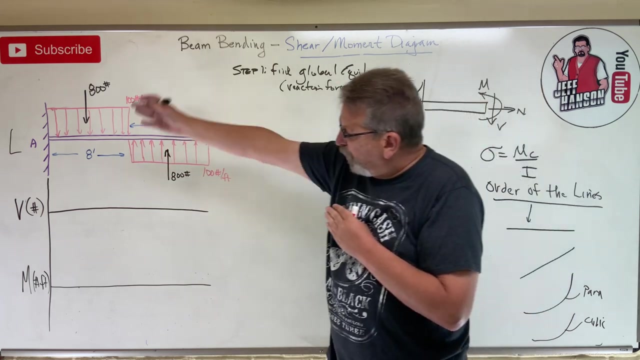 So, for all these problems, always okay, step one always is find global equilibrium, okay, Which really just means find the reaction forces, okay. So what do we have here? What kind of beam is that? What is that called? It's only hooked to a. 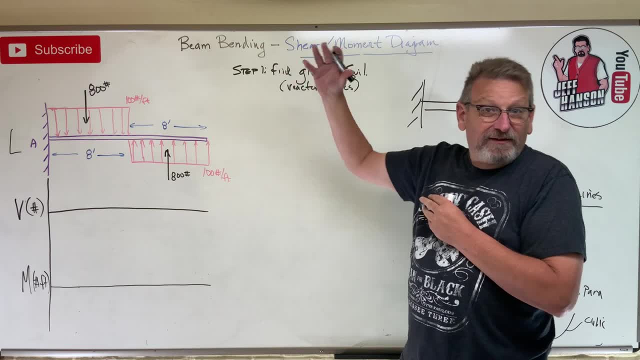 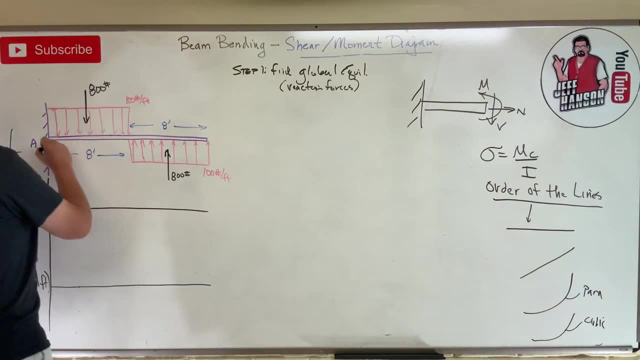 wall over there A There's no other supports on it. That's a cantilever beam right, Or a fixed support. What do you have there? Well, you have a reaction in the X, in the Y, rather AY, You have. 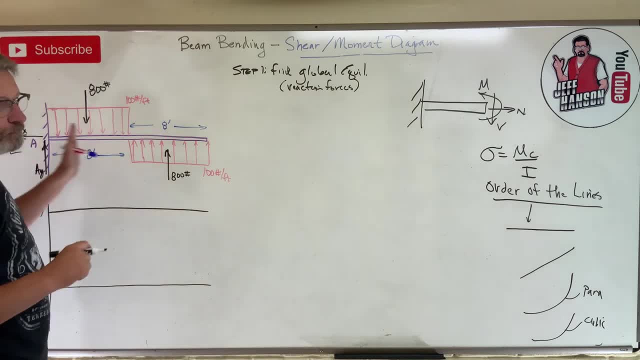 one in the X, I'll put an AX there. Of course, in this problem I have no forces in the X direction, So AX is going to be zero. And then you have some kind of a bending moment And I think all of this stuff here, oh, it may go that way, right. 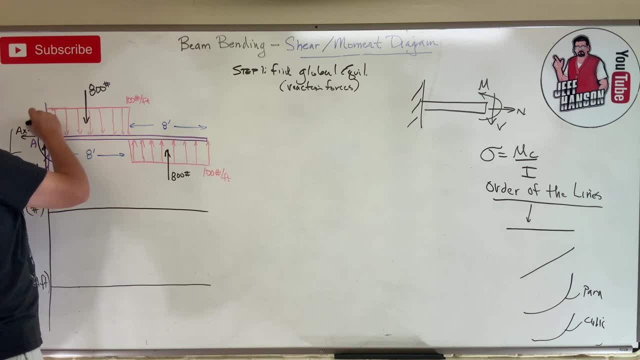 So I may have a moment like this, And I'm going to call him moment at A: okay, Why did you think it went up? Why did it go down? Well, because that force is the same as that one, but this one's. 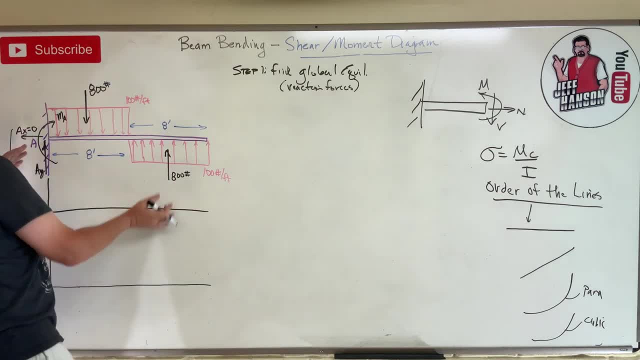 farther away. Force times. this is a moment. I think the net is going to be upwards right, And so I think this one has to counter it. That's what I. that's what I'm going to do, I think. I don't know if it's right or not. I'll find out here in a minute. I'm pretty sure it is. 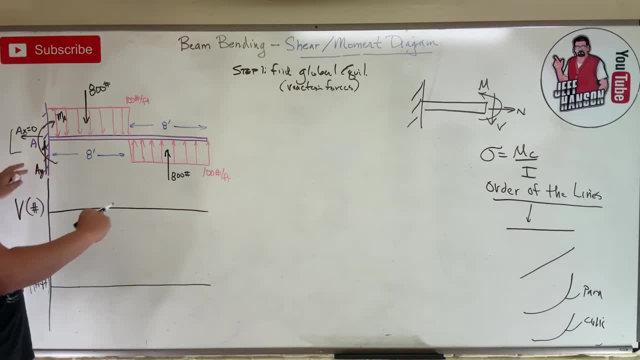 though. Okay, Now to find, oh to find. AY, I got to do some of the force in the Y, don't I? Well, I got 800 down, I got 800 up. So guess what some force in the Y is. 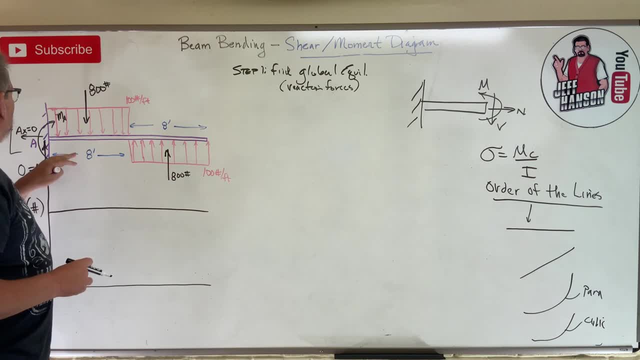 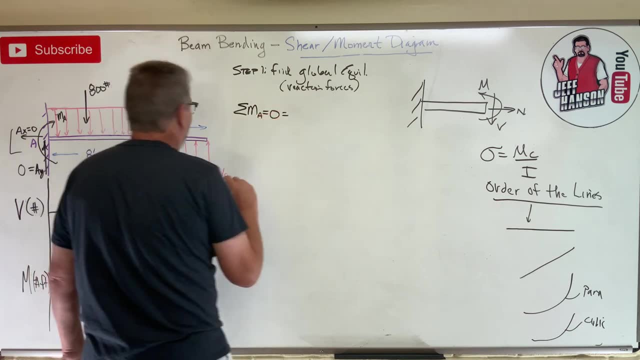 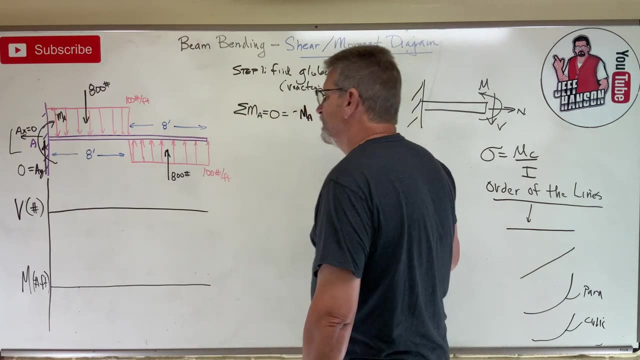 Zero. AY is zero. okay, How about MA? Can we find that Sum of the moments at A equals zero, equals what? Okay, MA, right, which I drew negative, So minus MA. And then here's 800, which also rotates me. 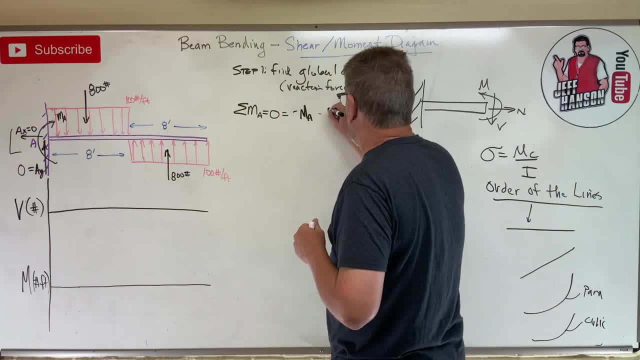 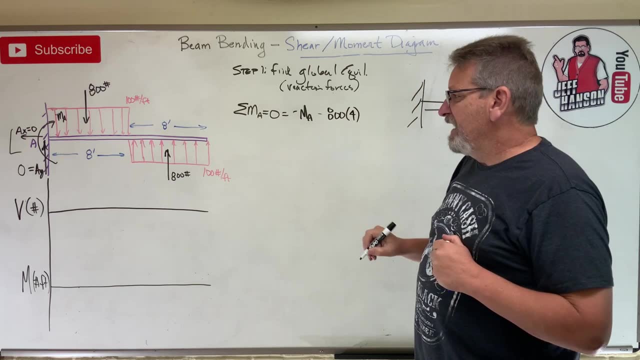 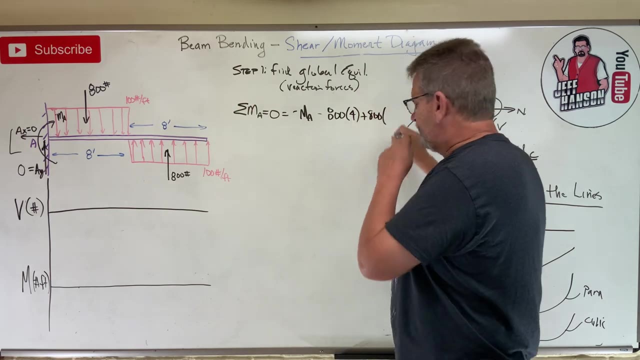 around point A negative. So minus 800 times how far away. Four feet, okay, Half of the eight right. And then I've got this 800, which rotates me the other way. So plus 800 times how far away. 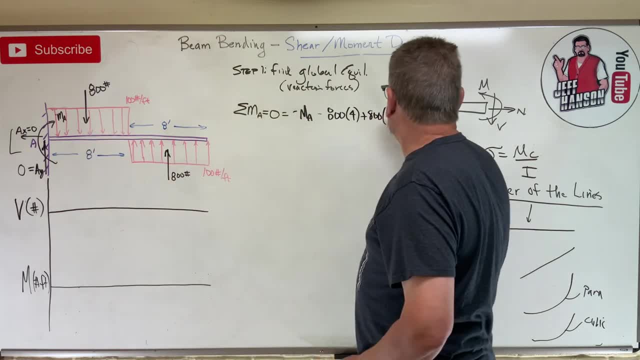 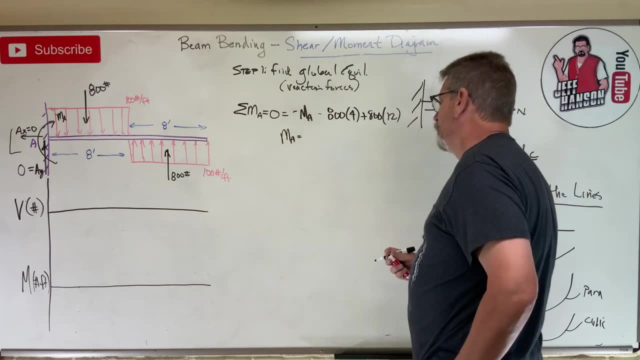 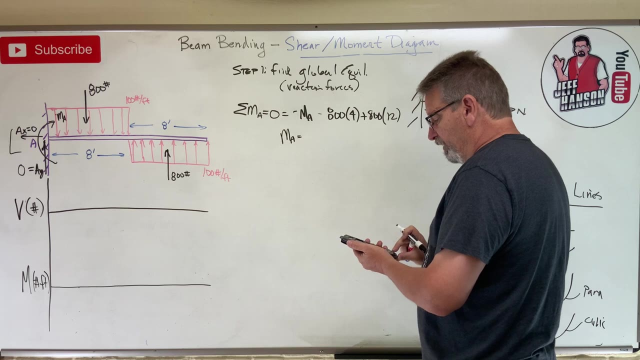 Eight plus another four is 12.. Okay, So I'm moving MA to the other side. That moment at A is equal to okay. how much is that? 800 times 12 equals 9,600 minus 800 times four: 6,400.. 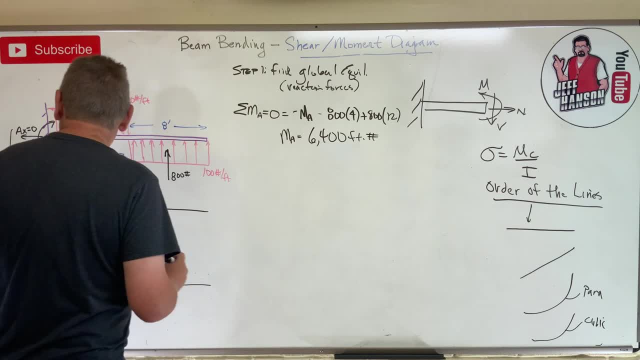 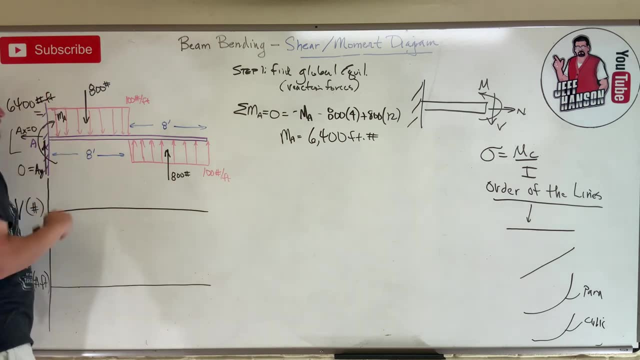 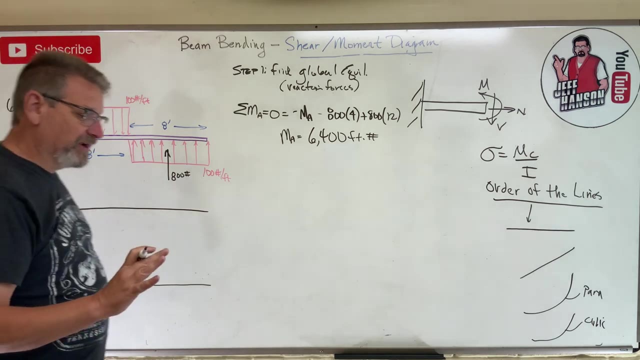 Pounds, okay. So that is this reaction over here at A 6,400 pound feet, okay, All right, I think that's it. Let's see if we can graph this Now, the first thing you got to do. 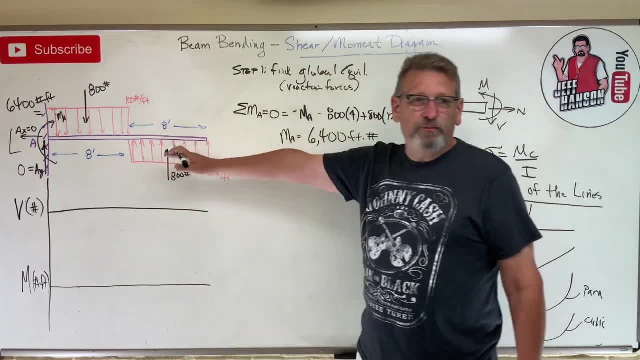 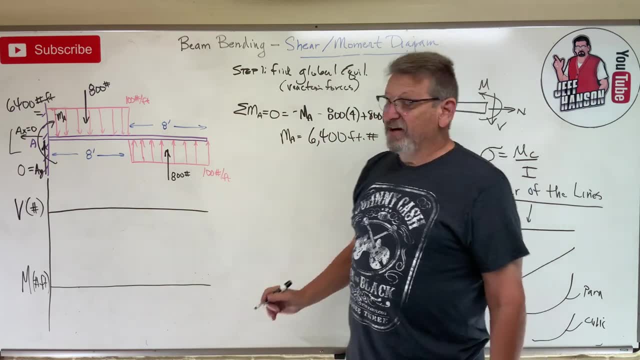 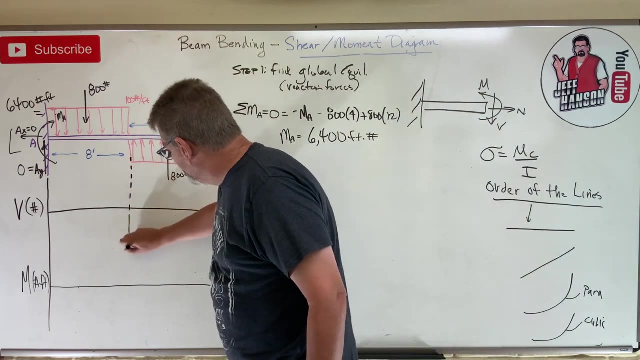 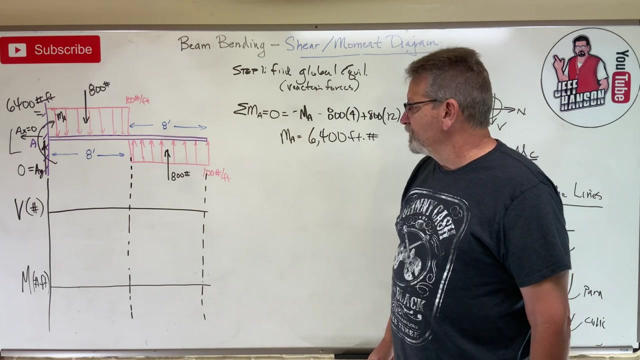 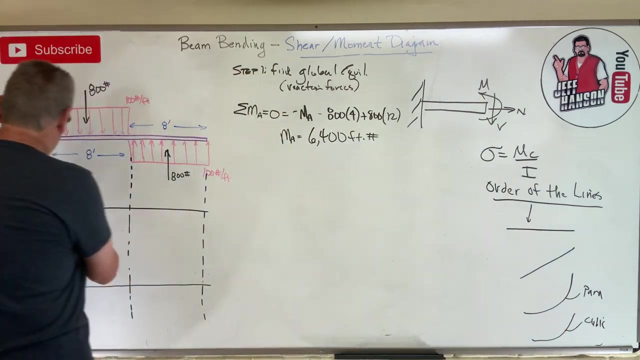 before you start graphing on these graphs is you have to add what are called discontinuities. A discontinuity is everywhere there is a change in the function And I just call it everywhere you go. So I'm going to start off at zero. okay, Now I don't have to do anything because AY is zero. 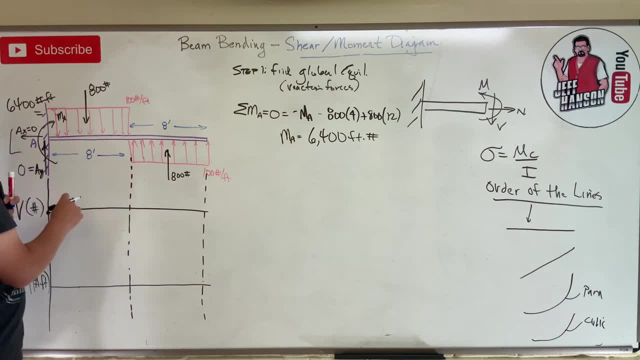 So it's not going to make me jump up or down. on my graph, This says: I'm going to start off at zero. I'm going to have to start. These arrows go downhill, don't they? So I'm going to go down. 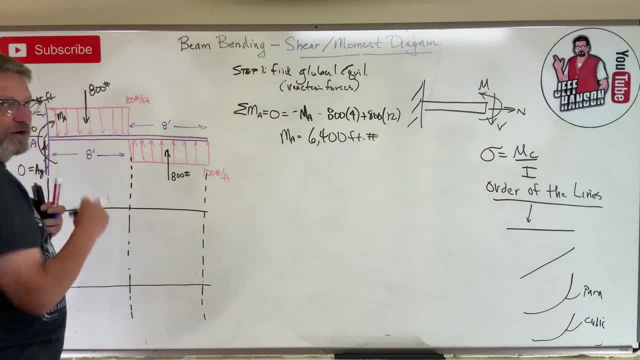 How much am I going to go down? Because I take a step, get 100 pounds. Take another step, get 100 pounds. So I like to think about it like this: You have a load backpack on your back, okay, You strap it on. There's nothing on there. You hop on the beam and you start walking across. 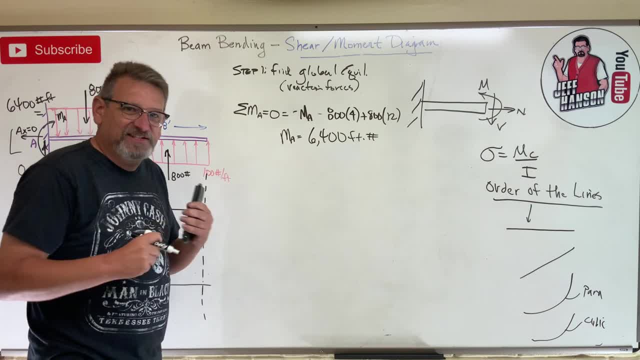 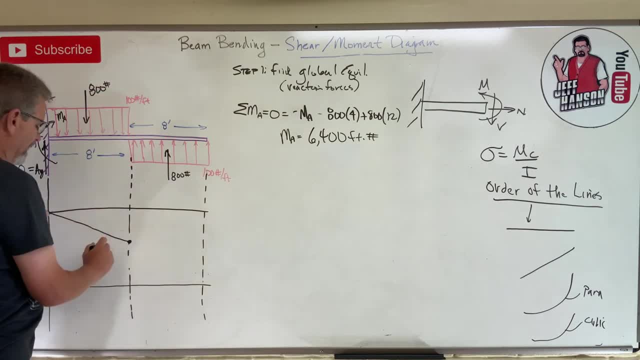 100 pounds. Bam, How much did I get? total: 800 pounds. okay, So there I am at negative 800, right Now, what's going to happen? Take another step. Somebody's putting 100 pounds, taking 100 pounds. 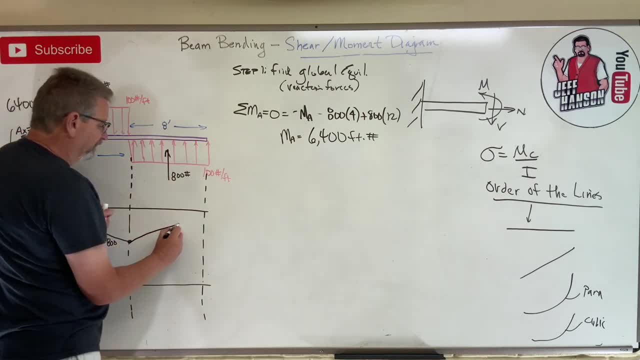 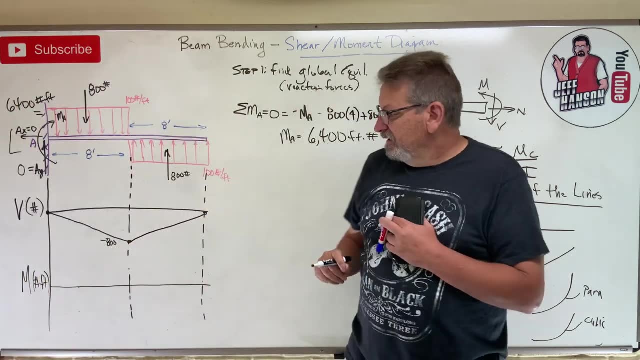 out of my bag, aren't they? 100 pounds, 100 pounds, 100 pounds. Take 800 out and bam Guess what. the sum of the forces for that whole beam need to be Zero. okay, Okay, Takes you right back to zero. 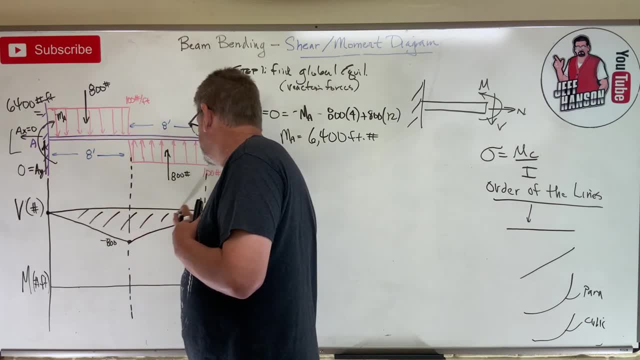 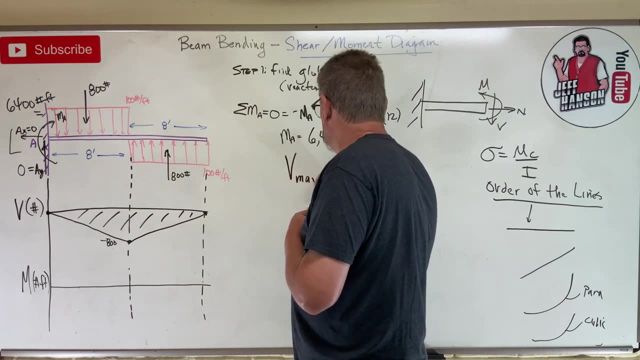 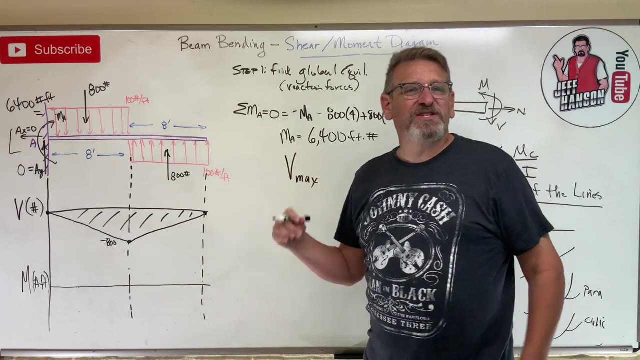 Zero again. okay, And there it is. okay. That's your V diagram. So if I ask you, what is V max? right, What is the maximum shear force? You're an engineer, You're designing a beam for me. That's the load that's on it. What's the maximum shear force you need to? 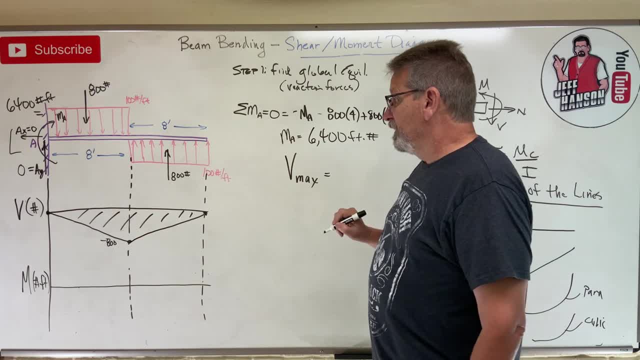 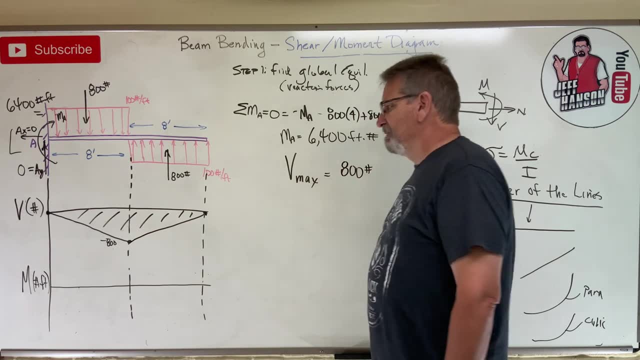 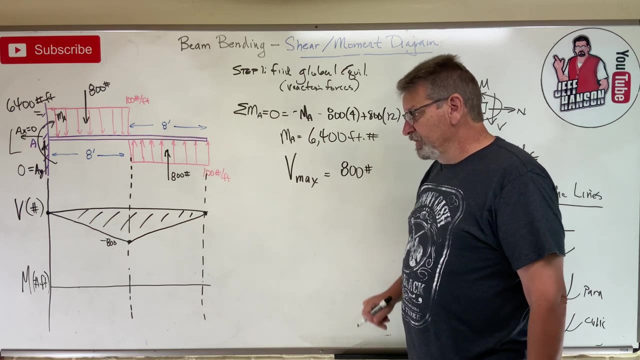 design for? Well, the answer is 800 pounds. okay, That's the maximum load on that beam. okay, Now let's go down and let's look at the moment. What's going to happen down here? So here's what I like to do on this Number one. this: 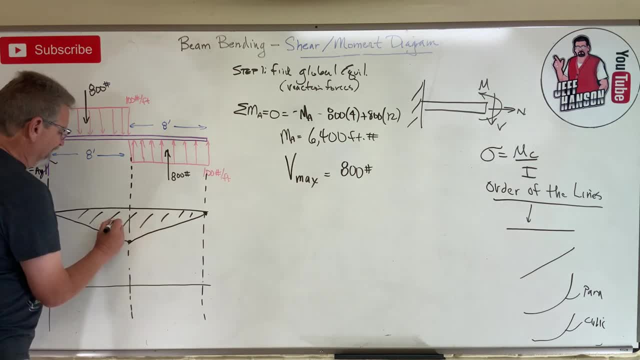 is called the graphic method. okay, I'm going to put a minus here and a minus there. okay, Because the minus means that I'm going to go on a slope down. If I have any areas that are above this axis, I'm going to put pluses on them, But this one's minus, So I'm going. 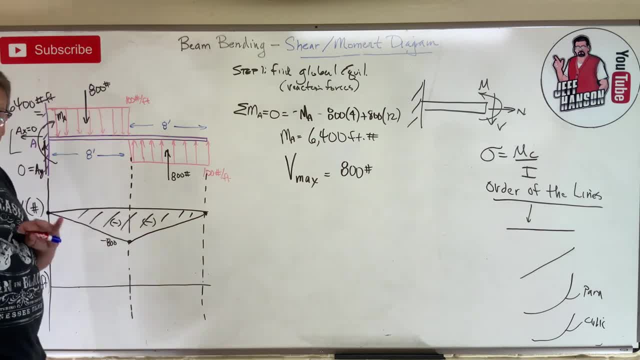 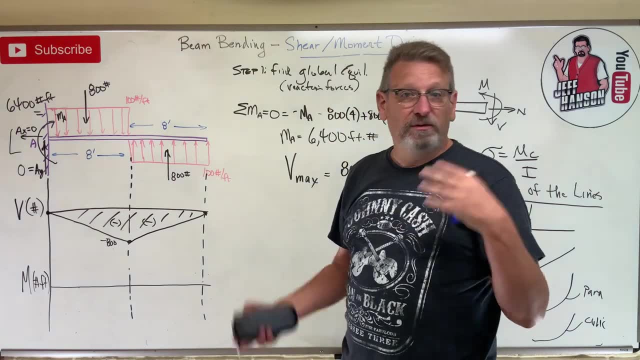 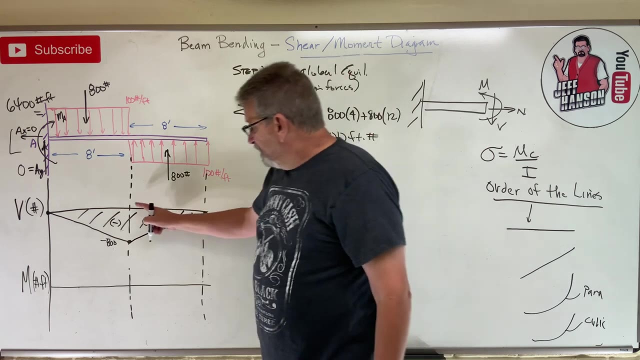 to put a minus and a minus. Now I know that the moment has to get back to zero. also, Shear moment graphs always have to get back to zero, always. If you don't get back to zero, you've messed something up. So that's your sign that I've messed something up Now. 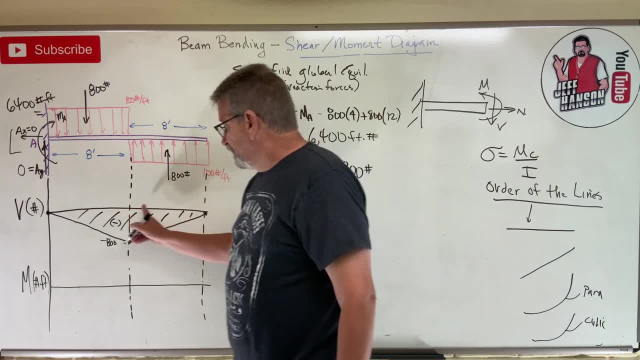 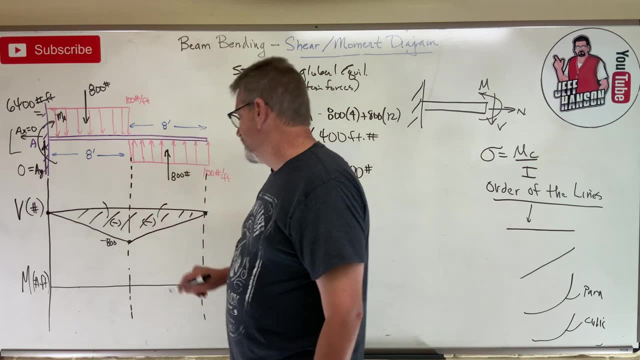 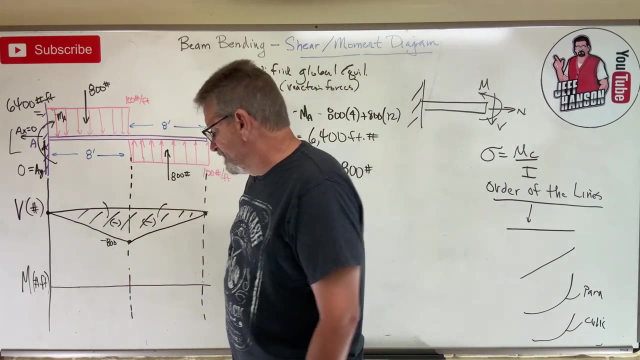 this value here is in pounds. This value here is in feet, right? So if I find the area of that shape and the area of that shape- they look the same, don't they- Then those units are going to be in pound feet. Hey, that's moment, okay. So the area. 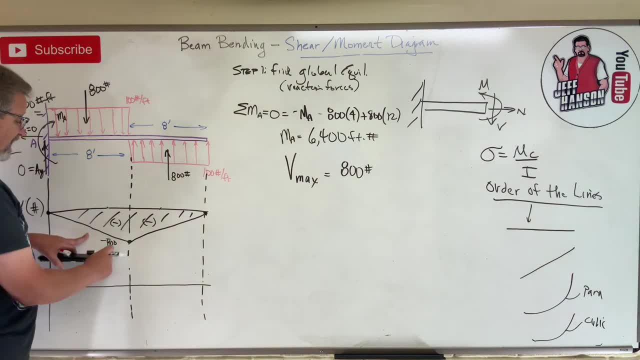 of this shape is what? So the area of this shape is 800 times 8.. That's 6400 divided by 2, because it's a triangle. So 3200 for you and this guy is 3200,. okay, Now the 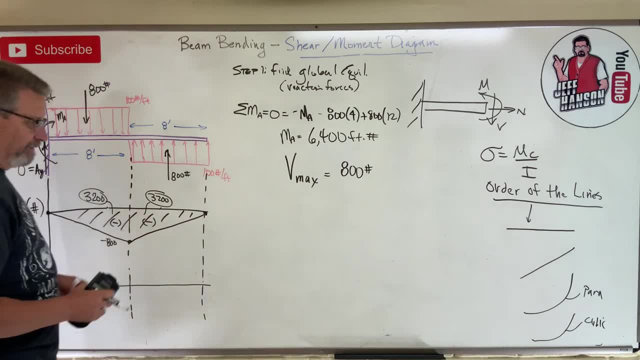 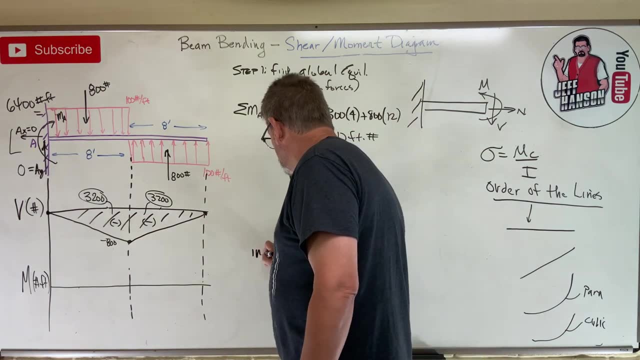 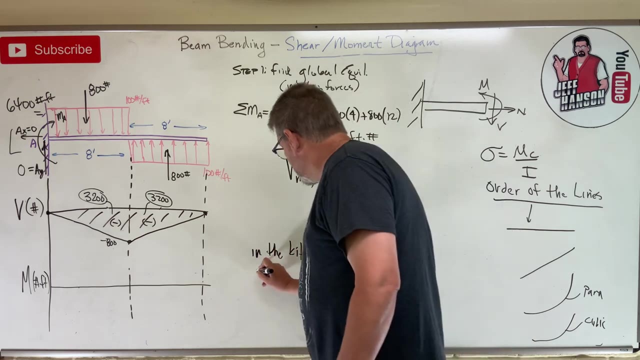 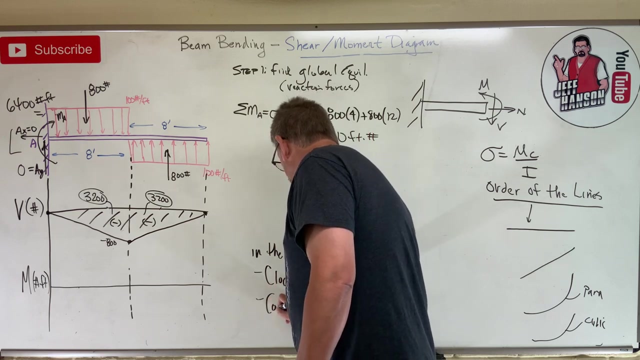 one we've got to watch for is this moment over here, because I've got a moment down here. How about a little funny saying: okay, to help you remember this. okay, How about this In the kitchen? okay, in your kitchen, check it out. the clock is above and the counter. 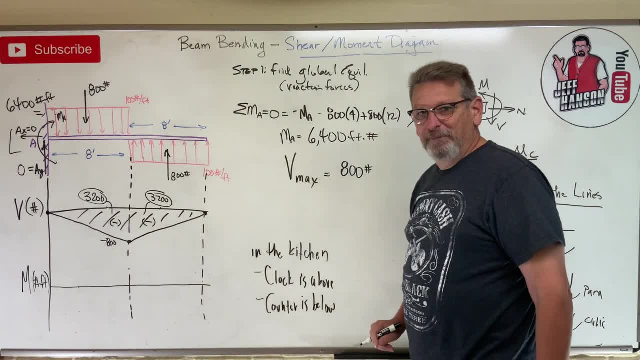 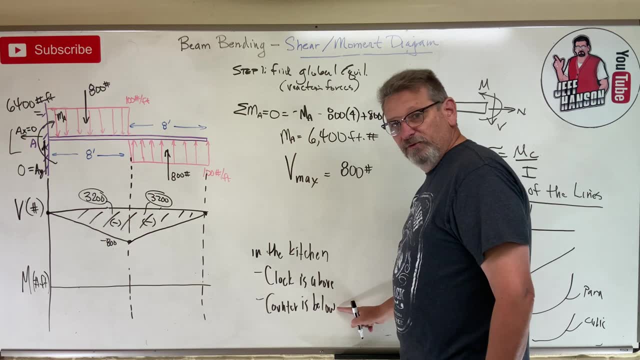 is below. okay, What does that mean? That if I have a clockwise moment, it's going to be above the axis. If I have a counterclockwise moment, it's below the axis. It's kind of silly, but I 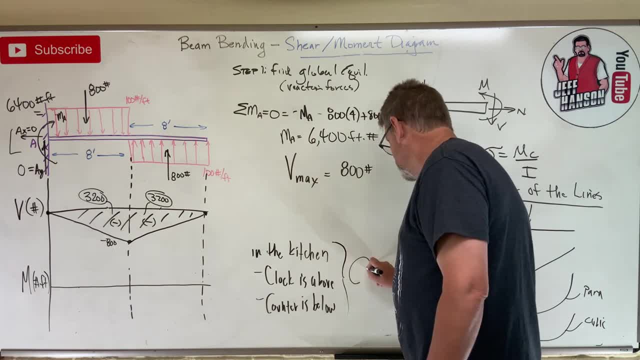 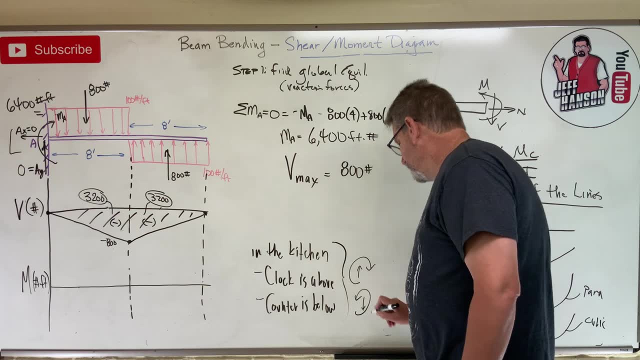 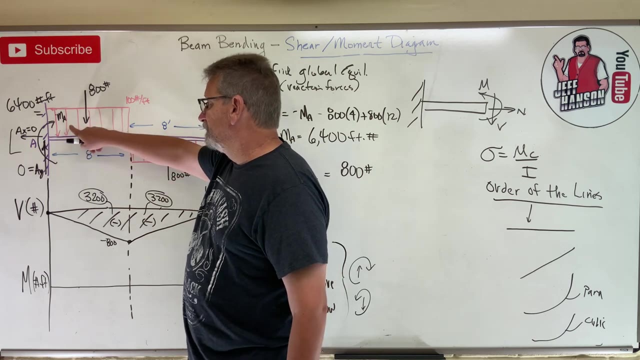 bet it'll help you, right. So, clockwise things that rotate me, like that, I'm going to go up. Things that rotate me counterclockwise, I'm going to go down. okay, Here we go, let's go. What do we have? 6400 is what. That's clockwise. so I'm going to go up 6400, okay. 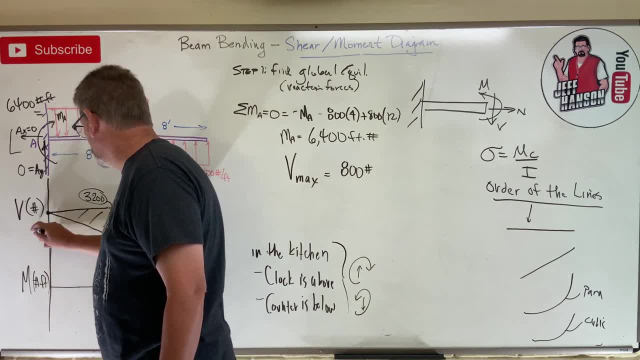 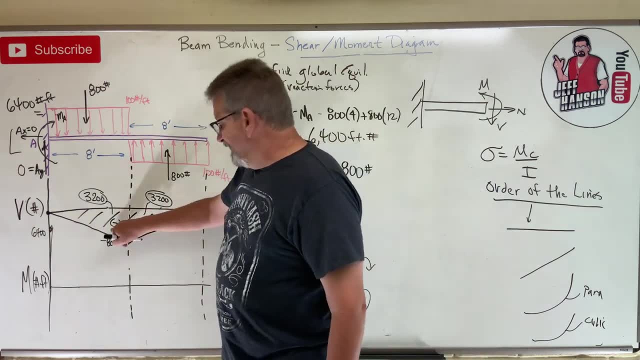 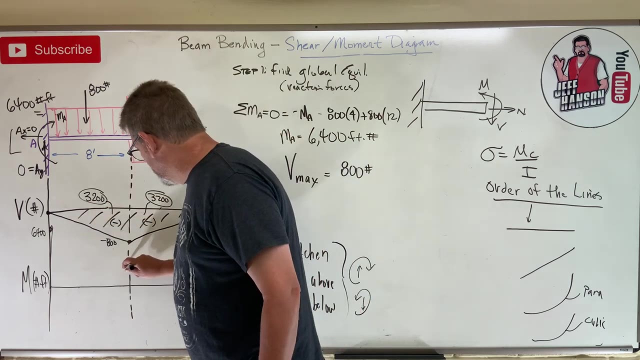 So here I go. There it is 6400, okay, And then what I'm going to go? I've got a negative, which means I'm going to go downhill. I'm going to go downhill- 3200, which is like halfway there. 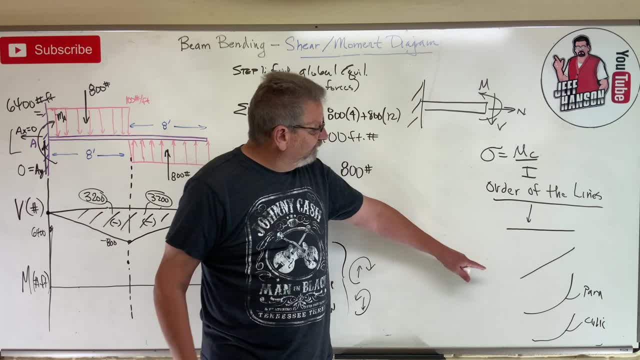 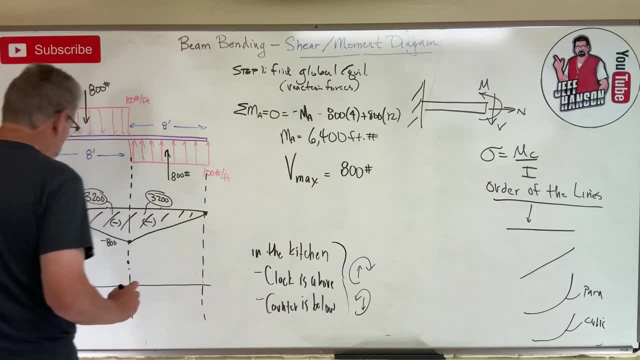 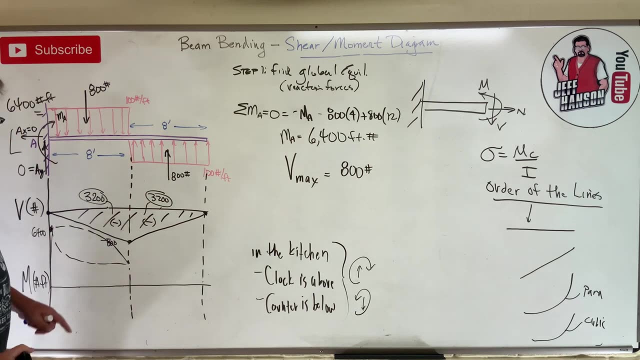 right From my order of the lines. I am here, I know it's going to be parabolic, and so you have two choices. That looks parabolic. That looks parabolic. Which one is the right choice? That's the question of the day. okay, Which one? Okay, the way I like to think about it is like this: 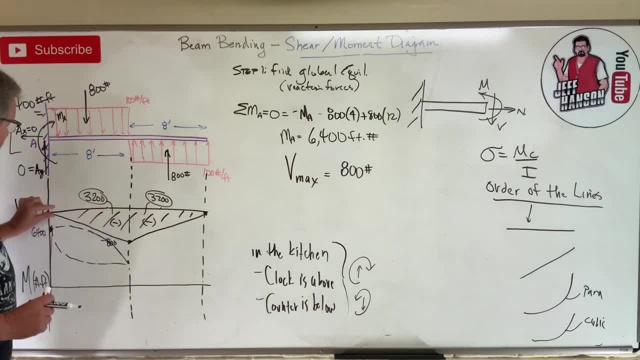 You're accumulating moment as you walk along the beam, but over here you're getting short stacks, short stacks. Take a step, get a little bit. Take another step, get a little bit. But over here, take a step, get a fat stack right. 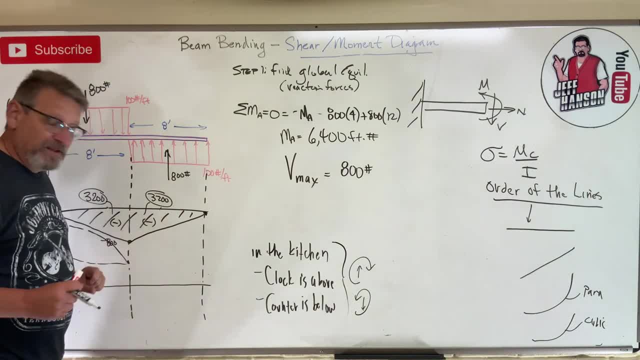 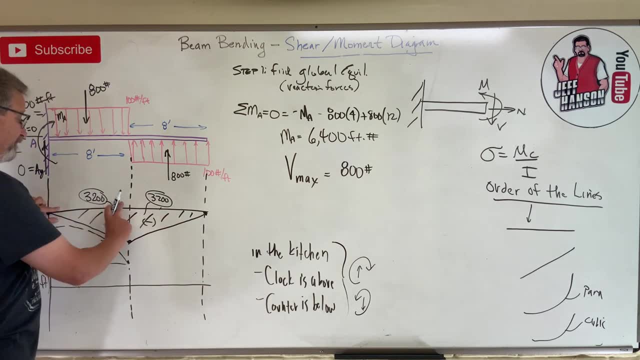 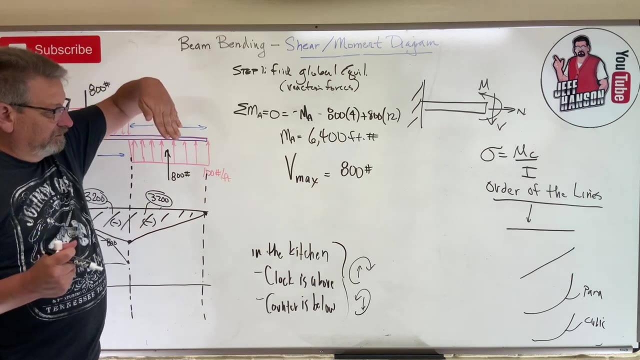 load. Slowly over here, but fast over there. The curve needs to follow that same thing. Fast then slow. Over here it's slow then fast. Think about snow skiing. right, What does a fast slope look like? That's a black diamond Straight down right. What does a slow slope look like? Oh, 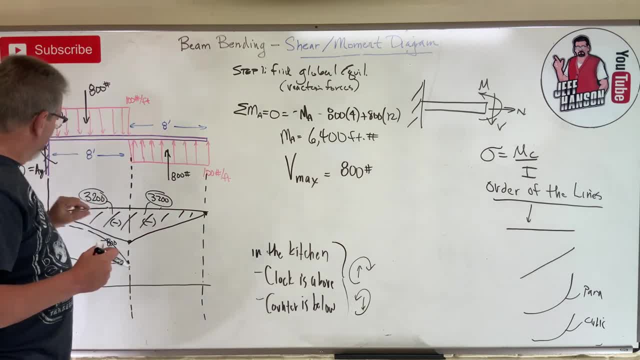 that's a bunny slope. It's almost flat, right. So if you're going slow, then fast. that would be flat, then steep. That would be this top curve, wouldn't it? It wouldn't be this one, It's going to be the. 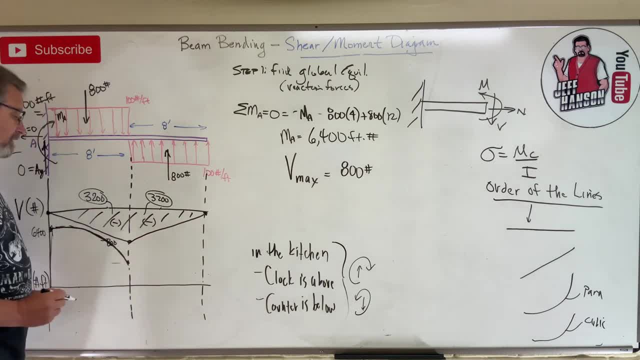 top curve. That one right there. okay, This works every single time. Now I'm at. I am at 3,200, but guess what? I got 3,200 more. Take me home to the place I belong on my moment graph back to zero. 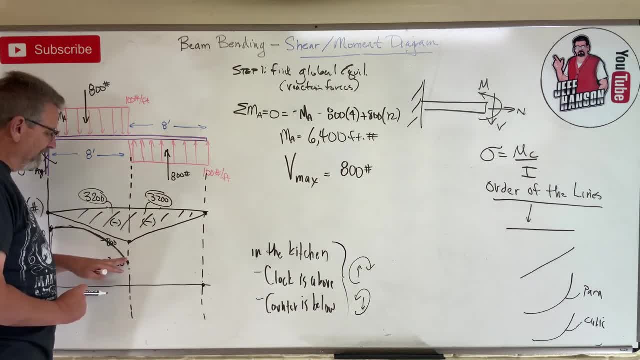 okay, How do I get there? How do I get from there to there? again Two choices: There's a parabolic this way or there's a parabolic that way. Which one is it? Well, over here I need to go fast, then slow. right, This one's slow, then fast, but this one. 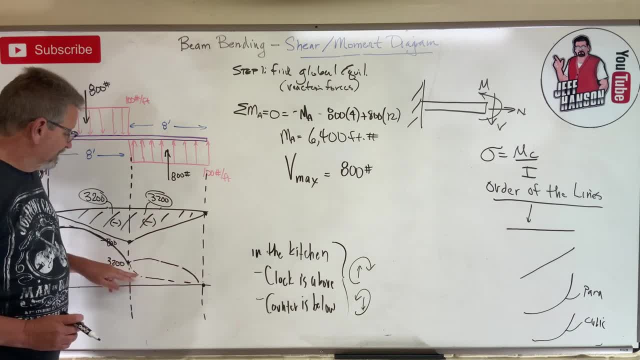 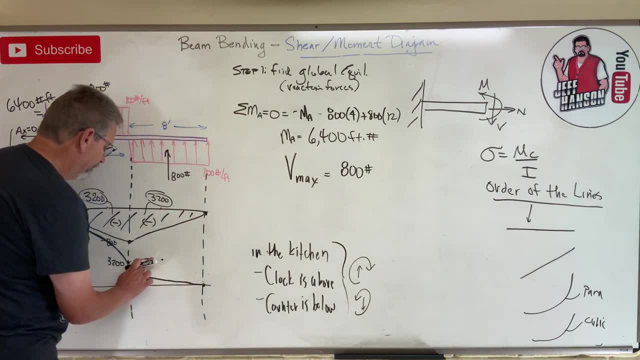 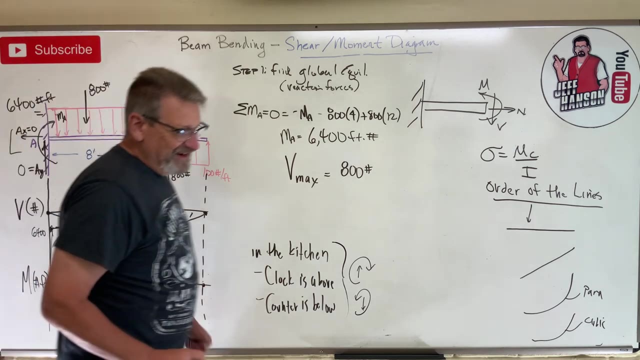 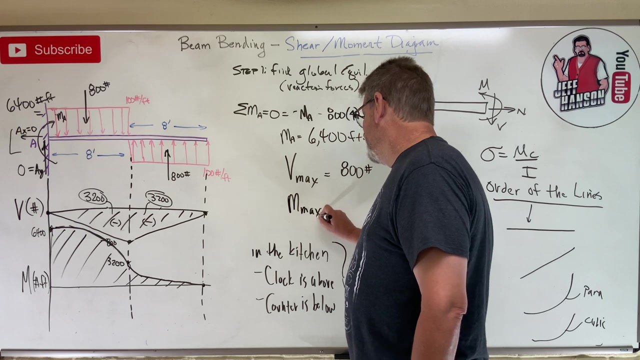 here is steep, then flat. That's the one I need. This is fast, then slow down here, isn't it That guy right there? okay, So here, bam, bam, bam, bam, bam bam is my moment diagram. okay, So if I ask you what is the biggest bending moment on that beam? 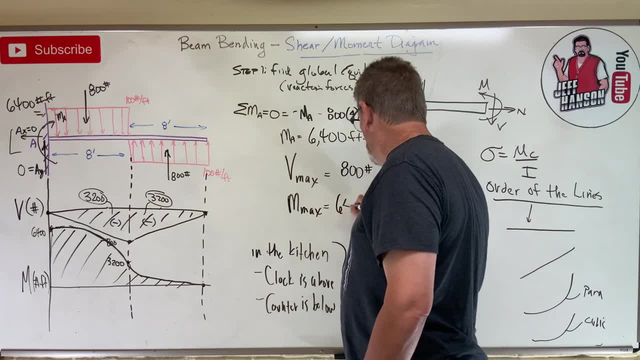 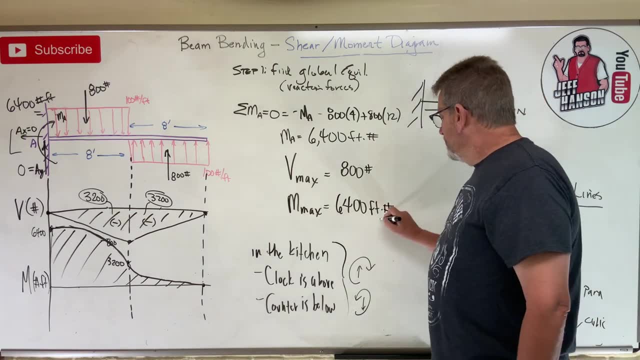 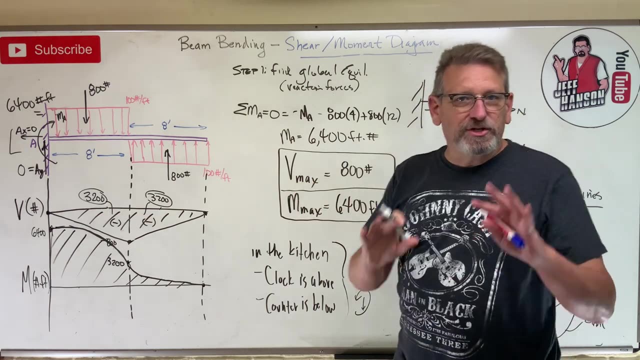 The answer is 6,400 foot pounds at that wall over there, isn't it? Okay, And that's the kind of information that I'm looking for on these graphs. okay, Now, that one was pretty easy. That was just a little starter, but I'm going to go ahead and do that. So I'm going to go ahead and do that. 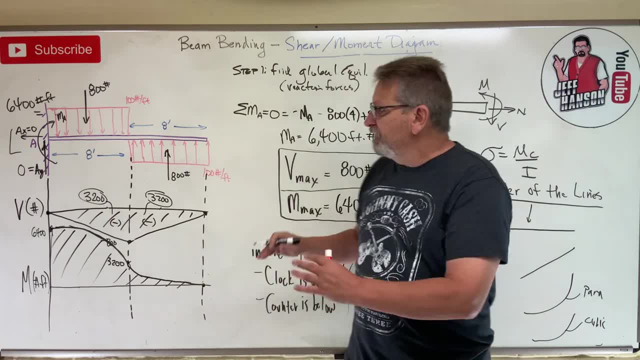 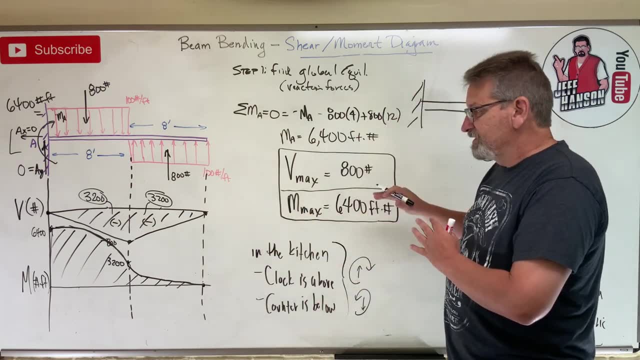 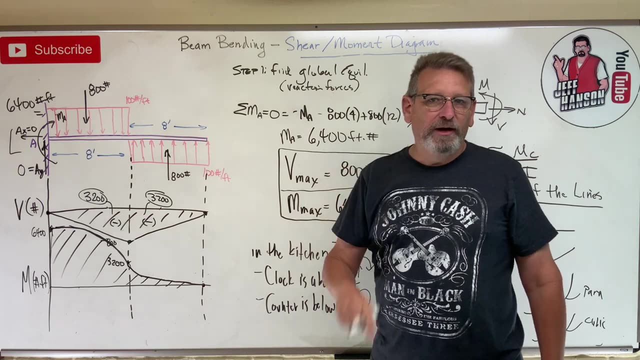 to get you introduced to the order of the lines and the fact that this and this and this are related with integrals, and then how to kind of approach this. okay, You know what? Let's work some harder ones. Let's go to the next video and see if we can't work one a little bit harder. I'll see you there.